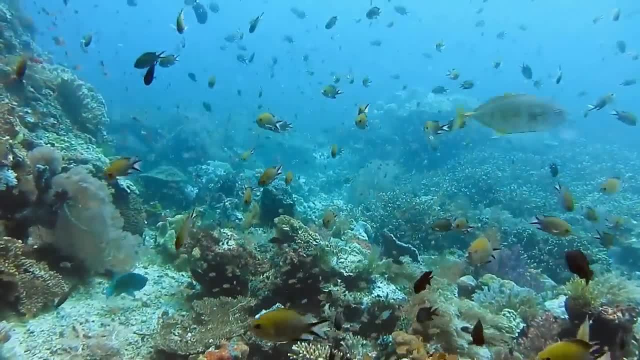 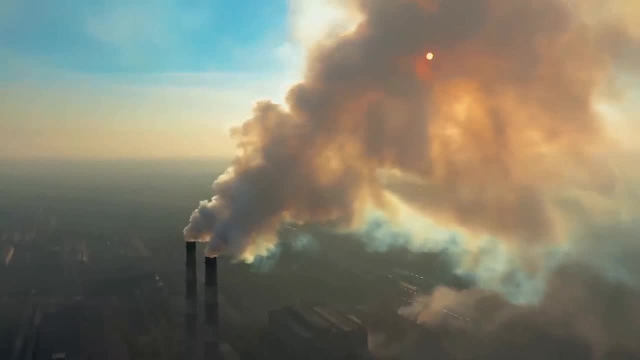 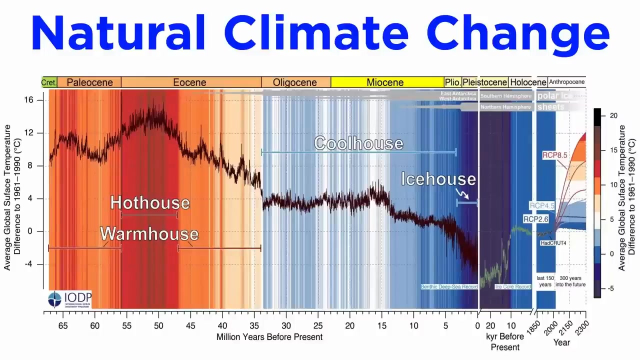 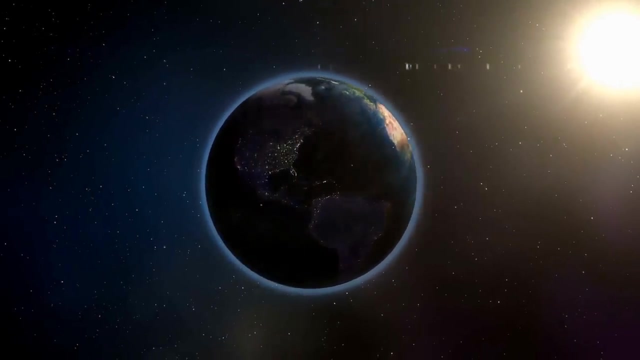 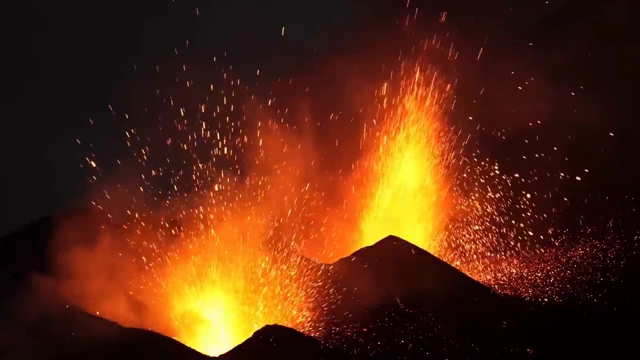 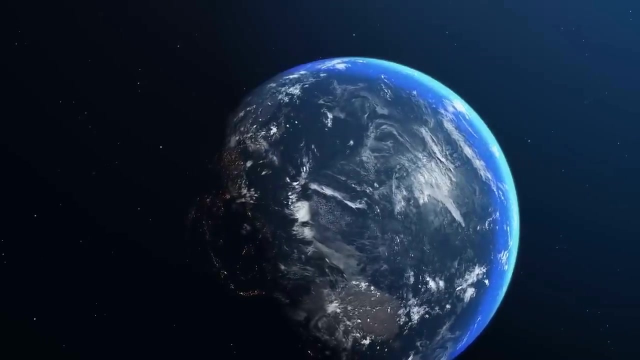 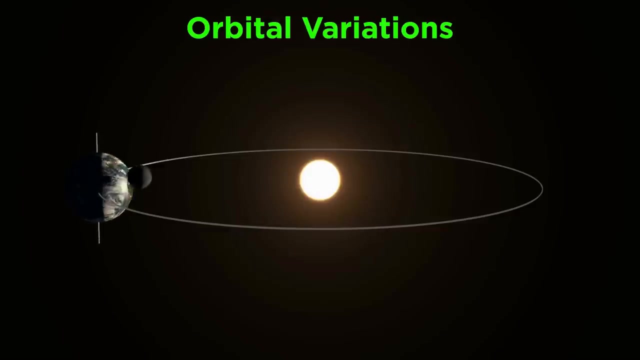 Previously we mentioned that the climate normals for the United States have been changed, and that organisms have specific environmental ranges that limit them to specific geographical regions. We will discuss human-induced climate change later, but we must recognize that natural climate change also exists. Throughout geological time, climate has changed naturally prior to human existence and influence. The natural variability and fluctuations of the climate system have always been a part of Earth's history. Natural climate changes can occur due to external variability, like changes in the Earth's orbit, or variations in solar intensity, but also due to internal factors, like volcanic eruptions or ocean circulation. Let's look at each of these factors now. First, let's discuss a familiar external factor responsible for natural climate change, orbital variations. The Earth revolves around the Sun in an elliptical orbit. However, its shape can vary slightly over time, sometimes becoming more circular and sometimes becoming more oval. This changes how much sunlight we receive on Earth, simply because there are times of year when the planet is closer to the Sun than other times. When Earth is closer to the Sun, it receives more solar radiation. The point at which Earth passes closest to the Sun is called the perihelion. 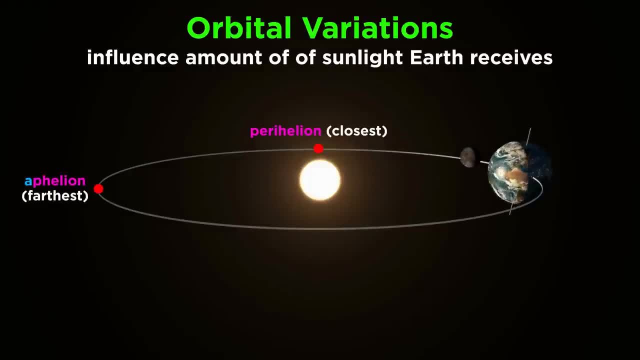 The point furthest from the Sun is the aphelion. An easy way to remember this is to think of A as in away, therefore the aphelion is when the Earth is furthest away from the Sun. 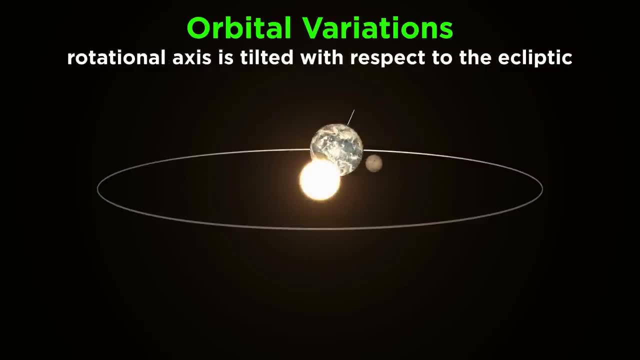 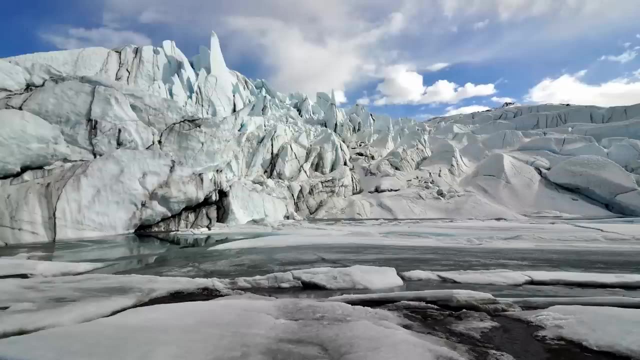 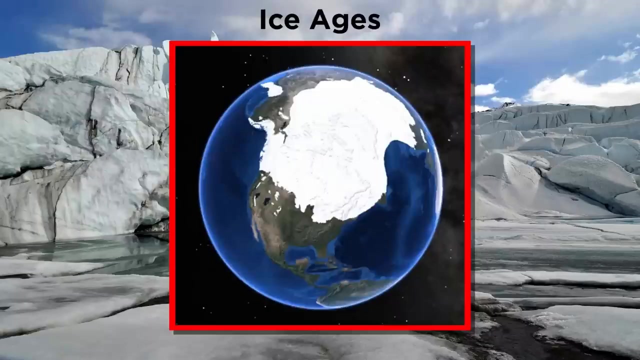 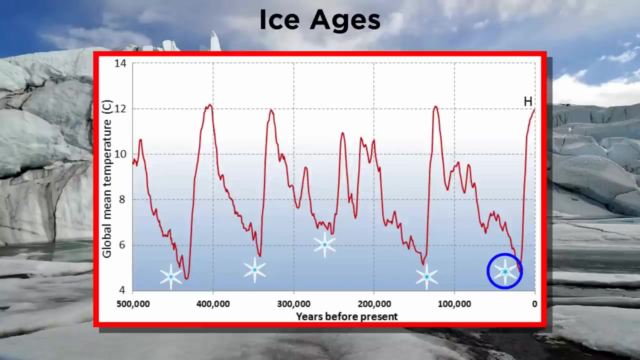 The Earth itself is also slightly tilted in terms of its rotational axis with respect to the ecliptic, or the plane of the solar system. The amount of this tilt changes with time, as does the direction of tilt, either towards or away from the Sun. These shifts and wobbles in Earth's orbit can trigger changes in climate, such as the beginning and end of ice ages, which are geologic periods during which thick ice sheets cover vast areas of land. To provide some context, the last ice age ended about 12,000 years ago, and the next cooling cycle may begin in about 30,000 years, if we were to make a prediction based on orbital cycles alone. 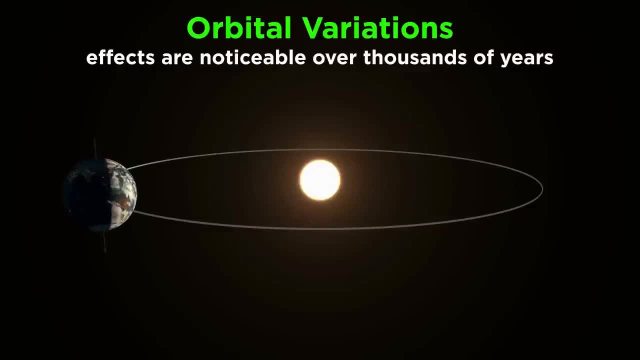 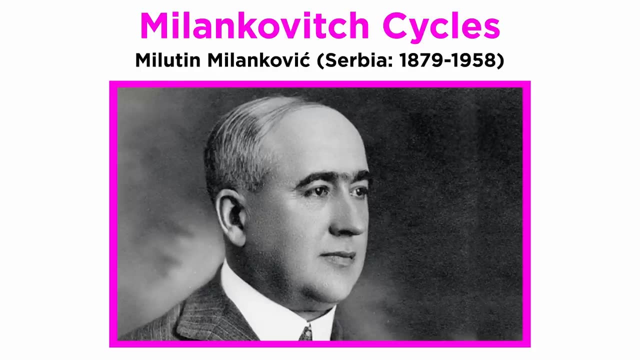 Orbital changes are so gradual that they're only noticeable over thousands of years, not decades or centuries. The collective effects of changes in the Earth's orbital movements upon its climate are called Milankovitch cycles, named after Serbian astronomer and geophysicist Milutin Milankovitch. There are several parameters that are relevant here. 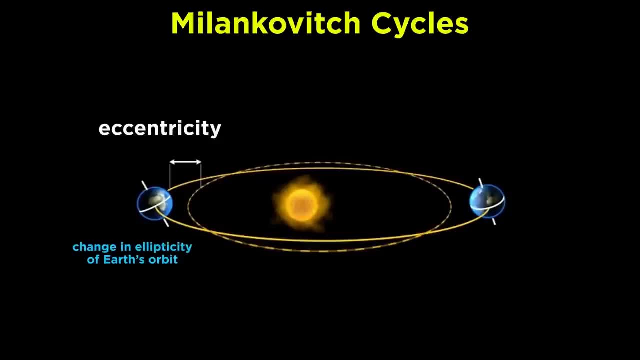 Eccentricity is the technical term used to describe how much the Earth's orbit around the Sun varies from more circular to more elliptical. This is due to the Sun and the gravitational attraction 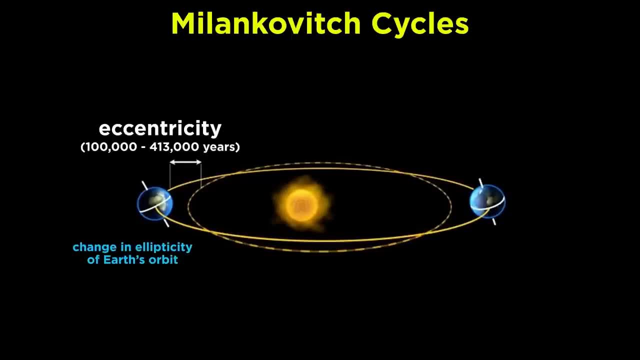 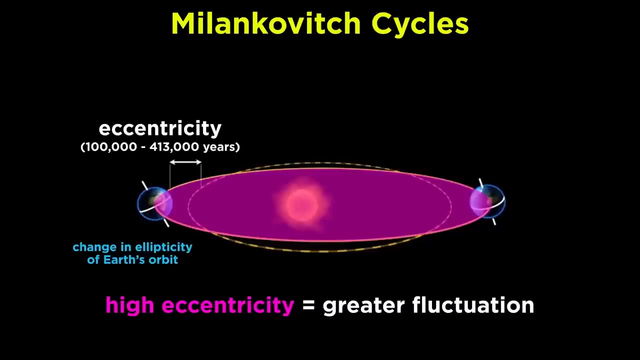 exerted by other planets. There are two periodicities, or cycle lengths, that have been identified. One cycle is an average of 100,000 years, and another, longer cycle is about 413,000 years. The average cycle is about 413,000 years, and the average cycle is about 413,000 years. The average cycle is about 413,000 years, and the average cycle is about 413,000 years. The average cycle is about 413,000 years. In periods of high eccentricity, radiation exposure on Earth 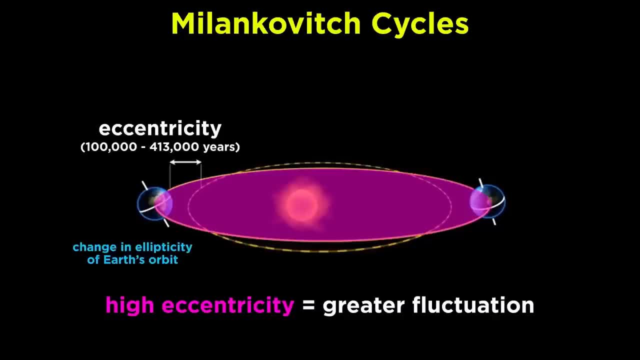 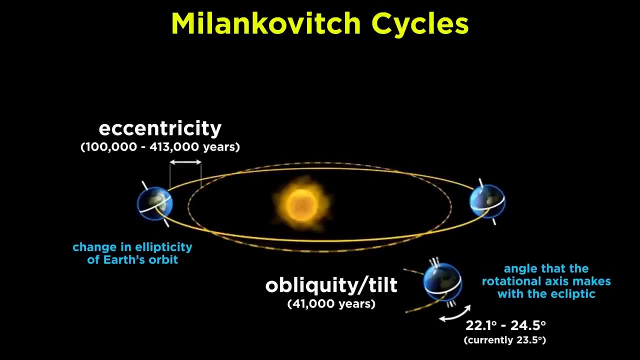 can fluctuate more wildly between perihelion and aphelion. Fluctuations are milder in terms of low eccentricity when Earth's orbit is more circular, leading to more stability in the climate. Obliquity is the technical term used to describe the tilt of the Earth. 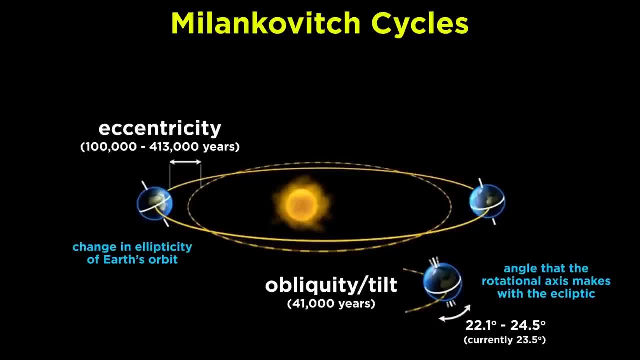 Currently, the Earth is tilted at 23.5 degrees to the vertical. This value fluctuates from 22 .1 to 24.5 degrees, which can lead to small but climatically important changes in the seasons. 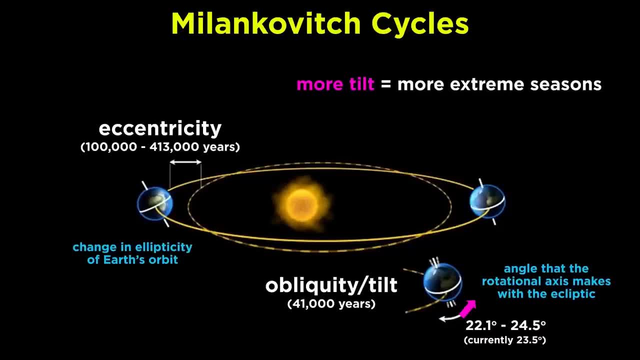 For example, more tilt means warmer summers and colder winters. Less tilt means cooler summers and milder winters. The periodicity of this change is on the order of 41,000 years. 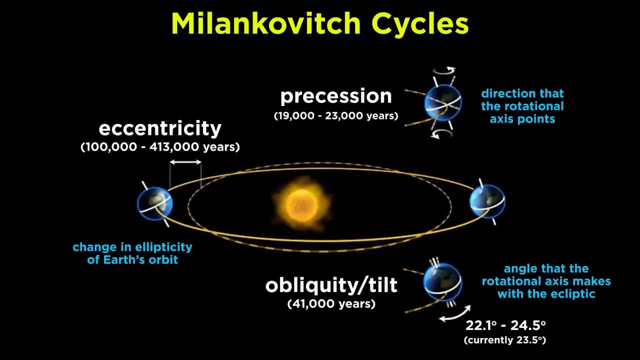 Finally, precession is the technical term for the motion of Earth's axis of rotation. It does not point in a fixed direction, but rather moves in a clockwise direction in space, like the spinning of a wobbling top. Of the three, 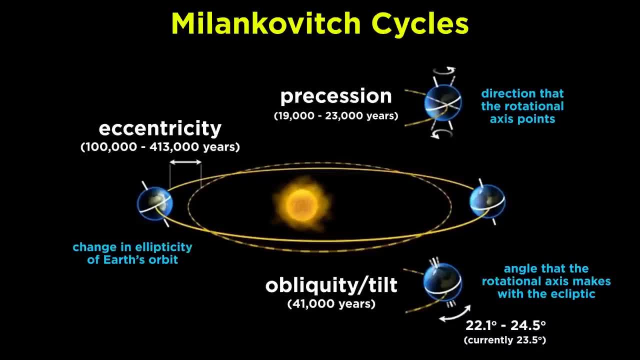 precession has the shortest periodicity, 19,000 to 23,000 years. 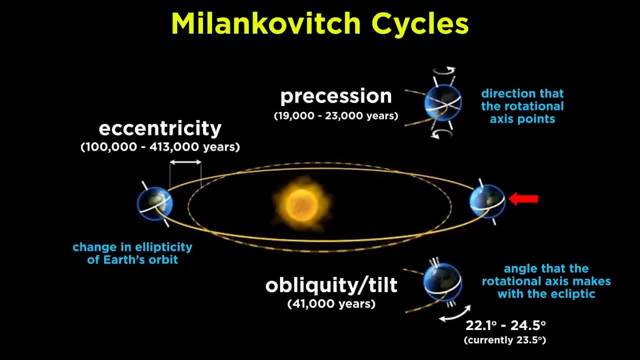 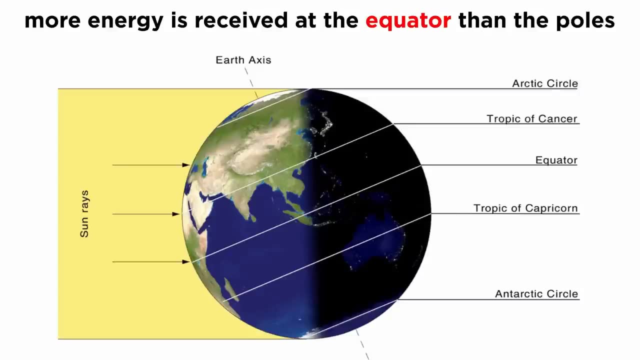 Solar radiation received at low latitudes on Earth is principally affected by variations in the cumulative effect of eccentricity and precession, whereas the higher latitudes are mainly affected by changes in obliquity. Since the Earth is tilted in its orbit, the regions of Earth do not receive 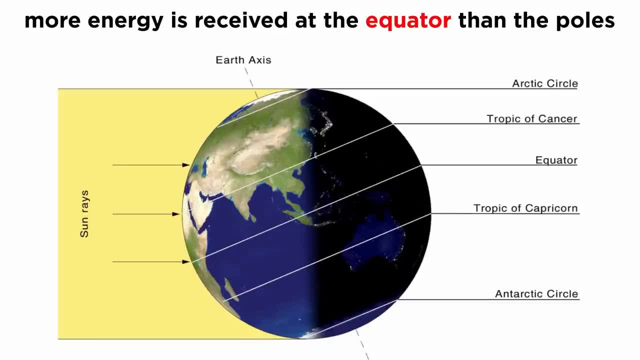 the same amount of energy, more energy is received at the equator than at the poles. 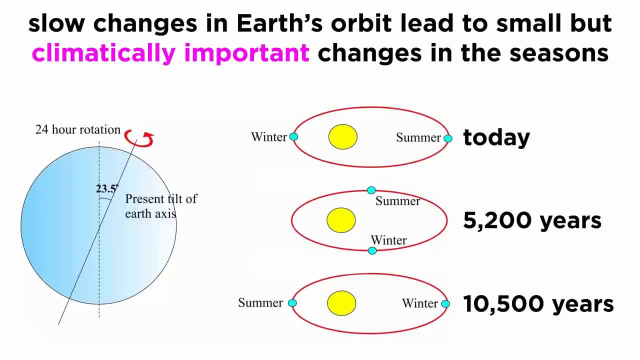 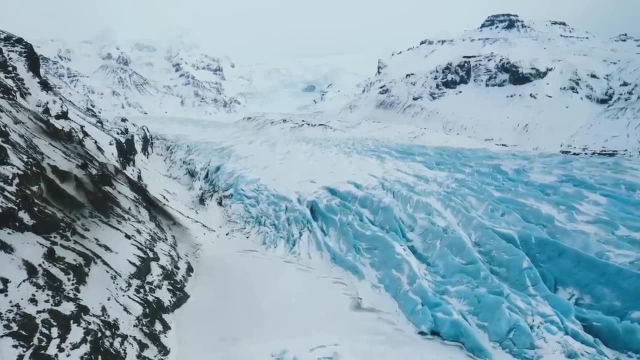 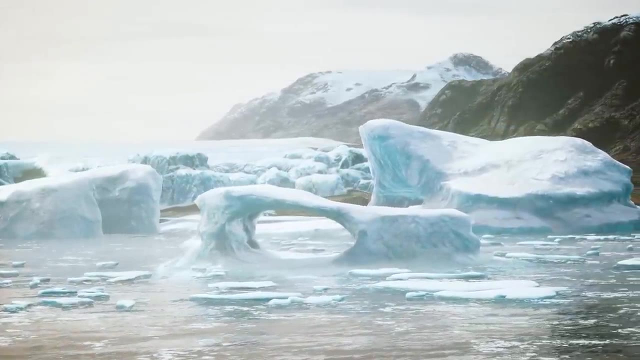 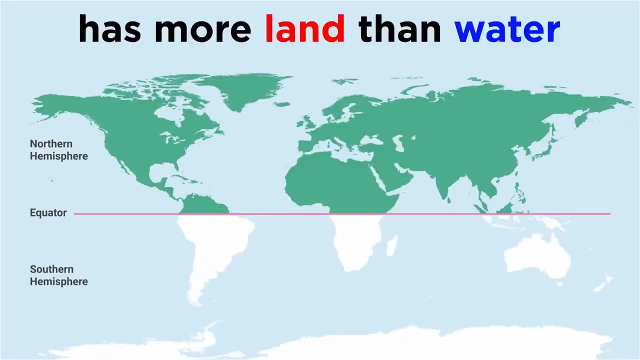 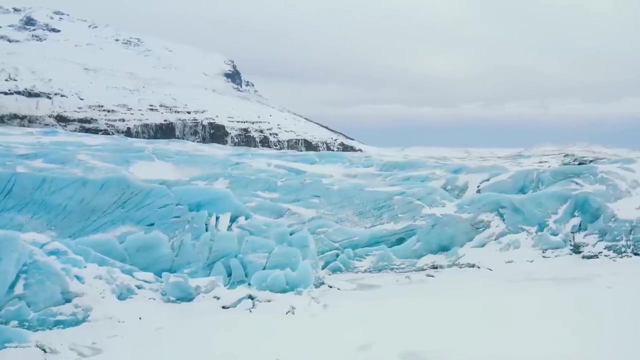 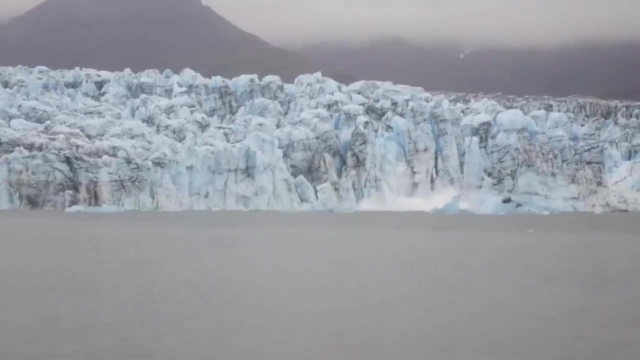 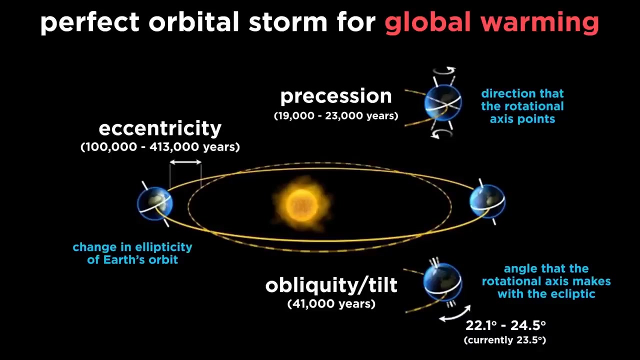 This difference can be exaggerated at different times. These slow changes in the Earth's orbit lead to small but climatically important changes in the strength of the seasons over tens of thousands of years. Additionally, other climate feedbacks in the internal climate system can amplify these small orbital changes. In the shift between glacial and interglacial periods on Earth, this is most related to the intensity of summers, in the northern hemisphere, which has more land than water. Land warms faster than water, so this hemisphere is typically more sensitive to changes in solar radiation. For example, when summers are mild, enough snow and ice remain throughout the season, maintaining glaciers and allowing them to grow larger in the winter. When summers are hotter, more ice melts in the summer than can be replenished in the winter, and ice growth is hindered. A perfect orbital storm, so to speak, for global warming. 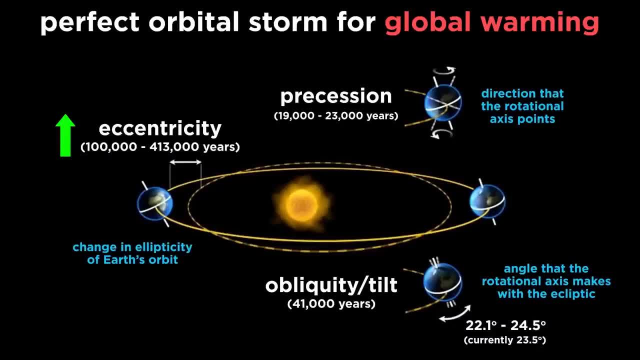 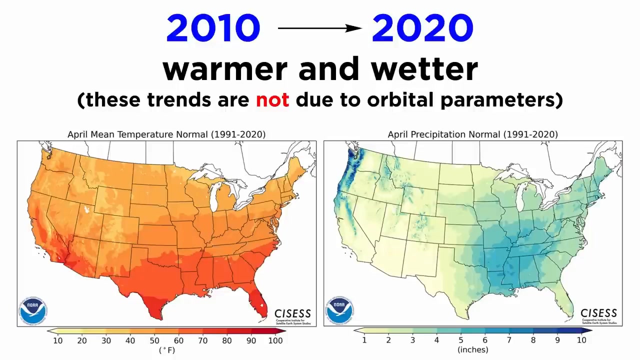 would require Earth's orbit at its highest eccentricity, Earth's axial obliquity at its highest, and the northern hemisphere in perihelion at summer solstice. Rather, in our current configuration, Earth's northern hemisphere currently experiences its summer in aphelion, the planet's obliquity is currently on the lower end, and the orbit is fairly circular. In fact, the current organization of Earth's orbital features should result in cooler temperatures, but instead the average temperature of the Earth's orbital features is lower. Thus, we cannot attribute current climate trends to orbital parameters. 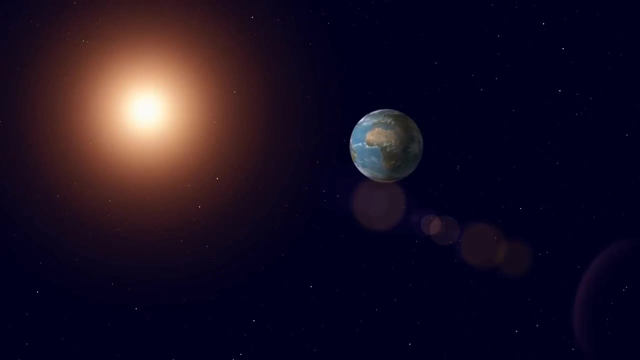 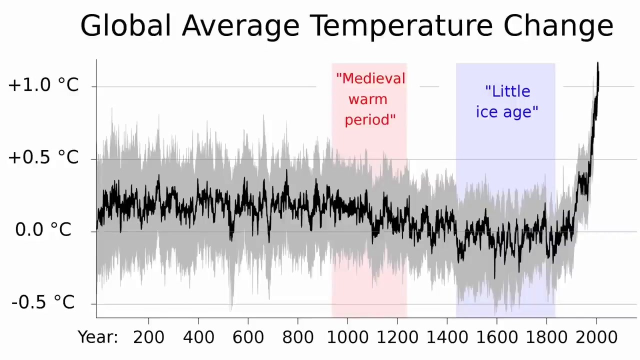 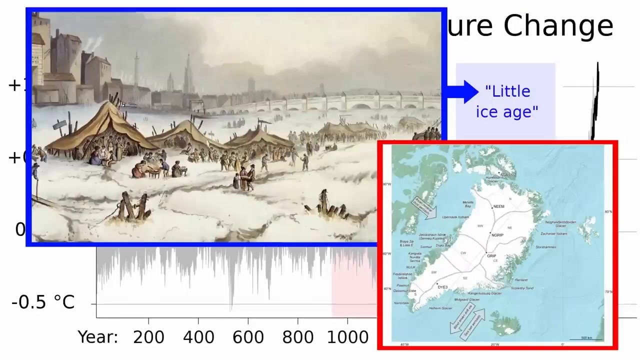 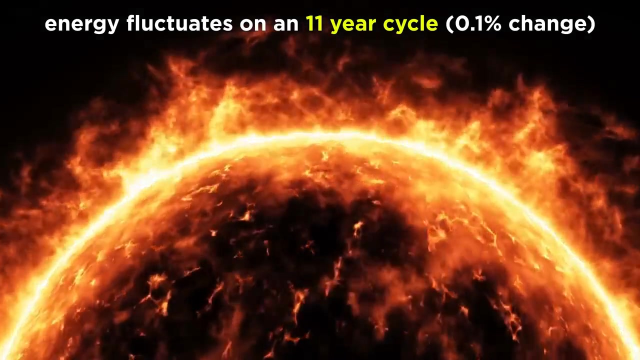 Let's also take a look at the sun itself. The sun is the source of energy for the Earth's climate system. Although the sun's energy output appears constant from an everyday point of view, small changes over an extended period of time can lead to climate changes. Scientific studies demonstrate that solar variations have played a role in past climate changes. For instance, solar activity was thought to have triggered the Little Ice Age, a cool period in the northern hemisphere between 1650 and 1850 when Greenland was largely cut off by ice, from 1410 to the 1720s, and glaciers advanced in the Alps. What about current global warming? The sun's energy fluctuates on a cycle that's 11 years long, and the energy changes only by about 0.1% during each cycle.